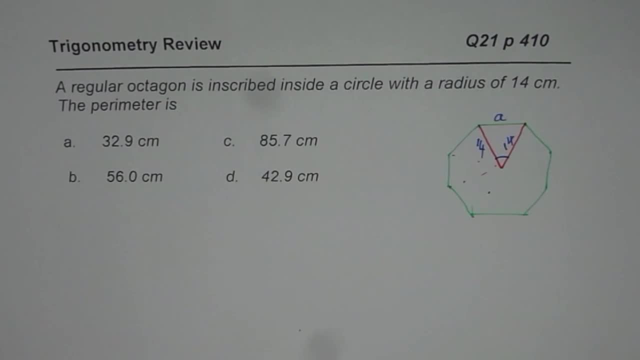 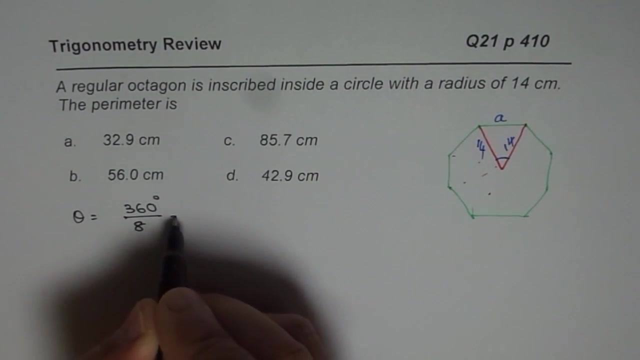 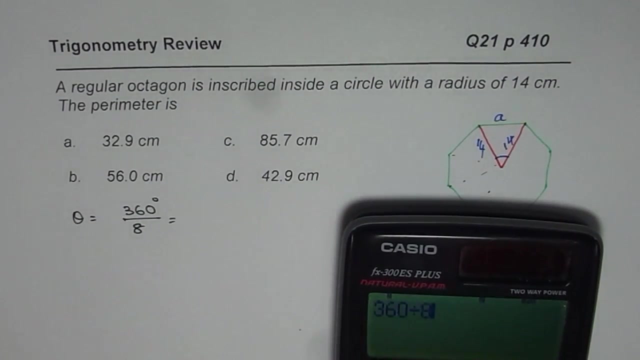 So let's find the angle. So let's find the angle first and then do the rest. Okay, so how do you find the angle of a regular octagon? Well, full angle is 360. So let's say angle theta is equals to 360 degrees divided by 8, right, Since there are eight triangles within this? Okay, so 360 divided by 8 is equals to 45 degrees. 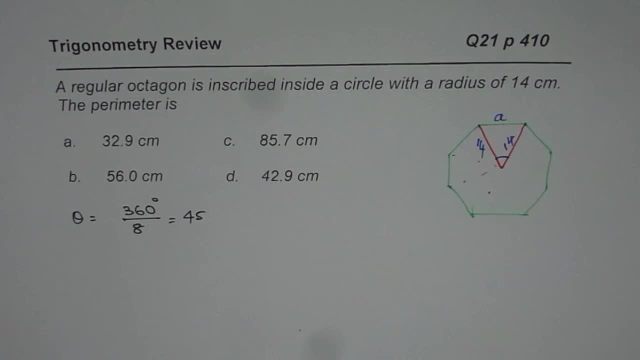 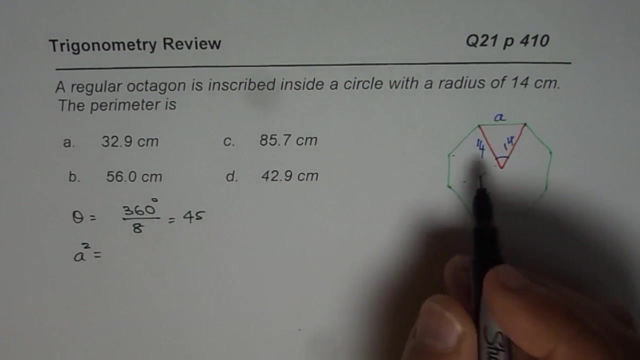 As the angle here. Now you can do a couple of things. One, since you know this is 45 degrees, you can use cosine law to find the side A right. So A will be. let me write A squared first. will be equals to 14 squared plus 14 squared minus two times both the sides right. 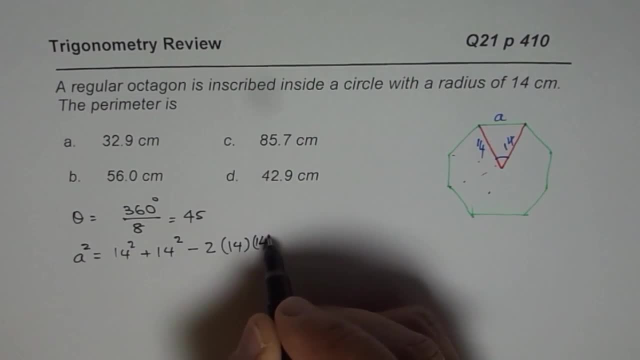 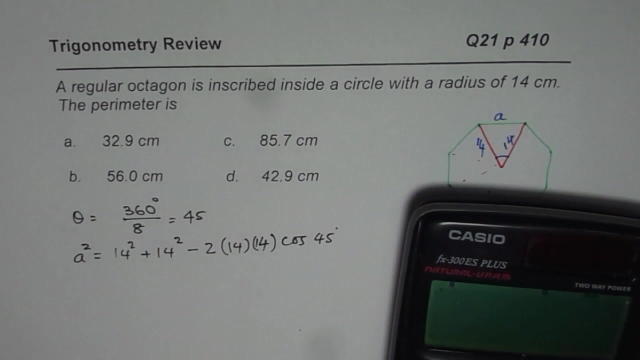 14 times 14.. Times cos of the angle within which is 45 degrees, right, 45 degrees. So this is one way of doing it. So let's calculate and then we'll find the answer. We'll multiply this by 8, correct? So we have 14 squared plus 14, squared minus two times 14 squared cos of 45 degrees is equal to how much? 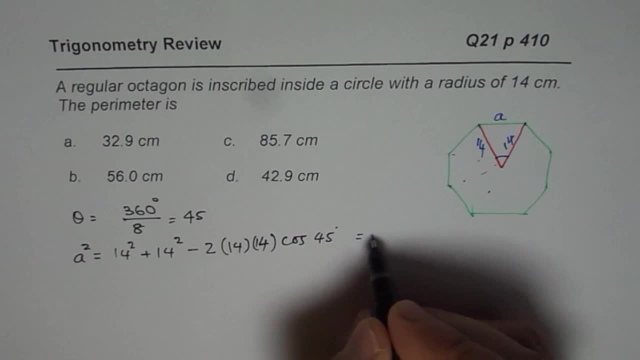 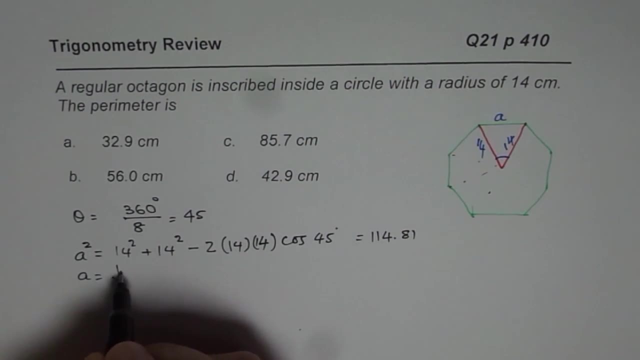 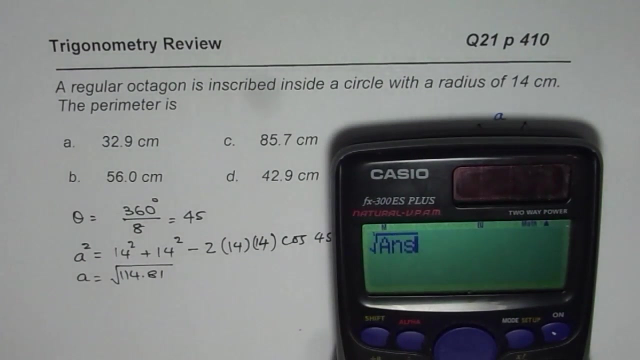 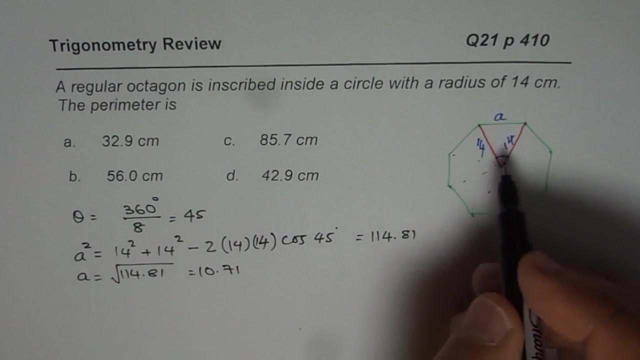 114.81,. right, So it is 114.81.. Now we can do square root of this to get A. So A is equals to square root of 114.81,. right, So that is square root of the answer equals to 10.71.. So it's reasonable, right? 10.71 is reasonable. It looks to be lesser than 14.. Okay now what is the perimeter? 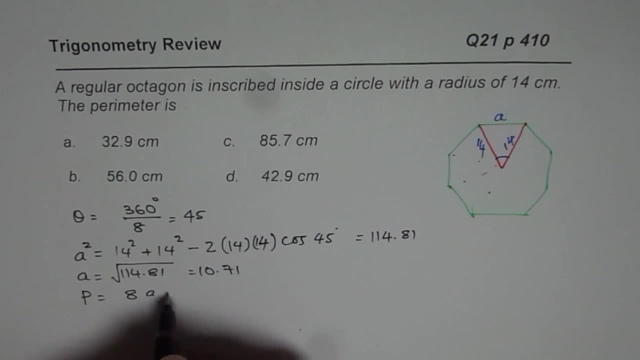 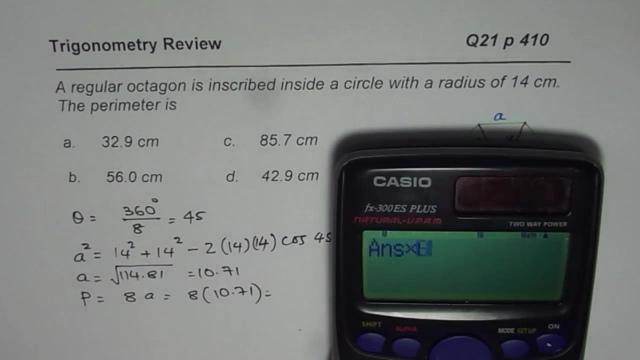 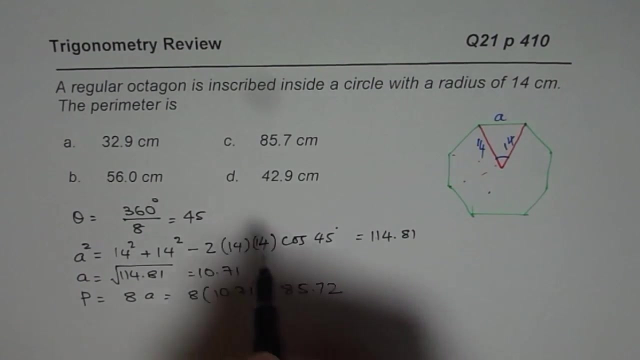 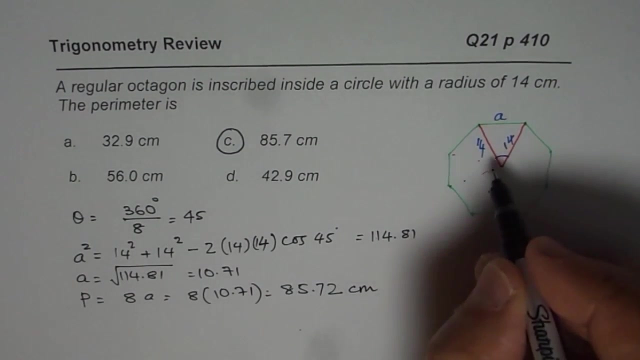 So we get perimeter as 8 times A. So it is 8 times 10.71.. Let's multiply this 10.71 by 8 to get the answer 85.72.. So 85.72.. That matches with option C. So that is how you can find the answer right, And of course it has to be in centimeters, since all these units are in centimeters, right? So that's the way to do it. I hope it helps. Thank you and all the best.